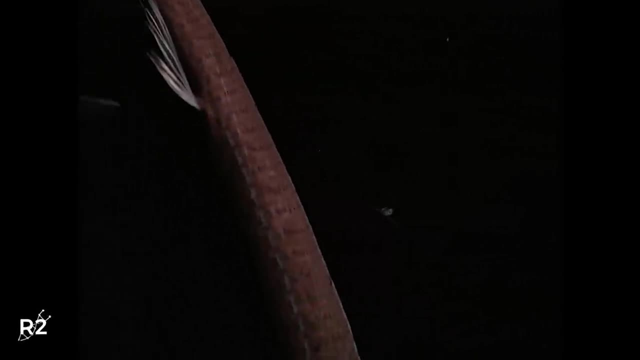 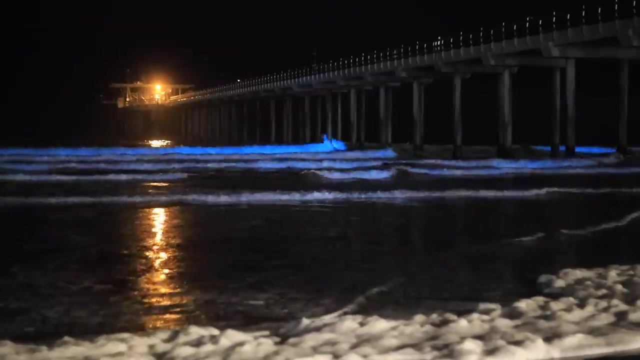 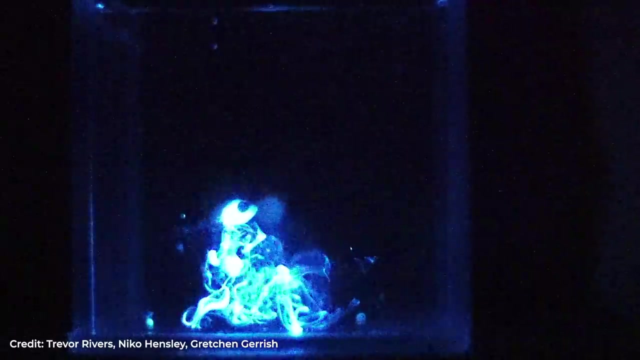 making it an impressive example of convergent evolution. And if you consider that 71% of the earth's surface is water, that means bioluminescence is actually one of the most widespread traits to have ever evolved. But that also raises the question: why is bioluminescence so common in the ocean and so rare on land, The only terrestrial 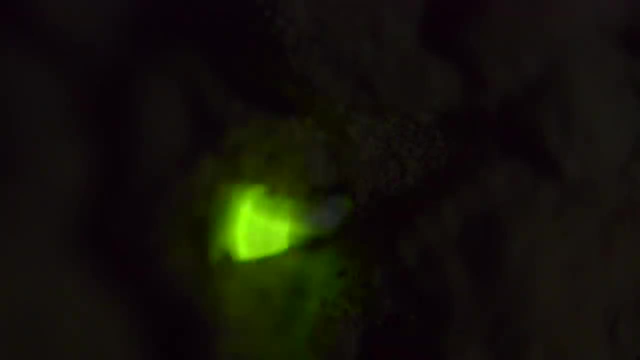 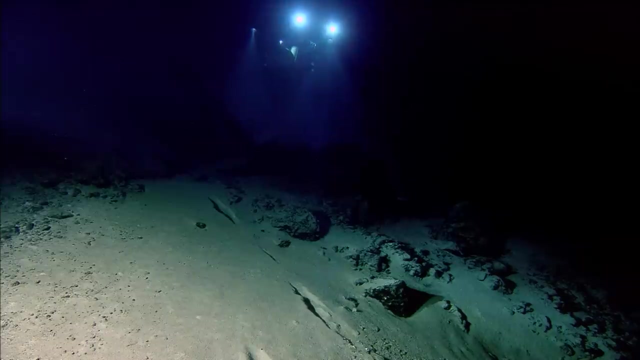 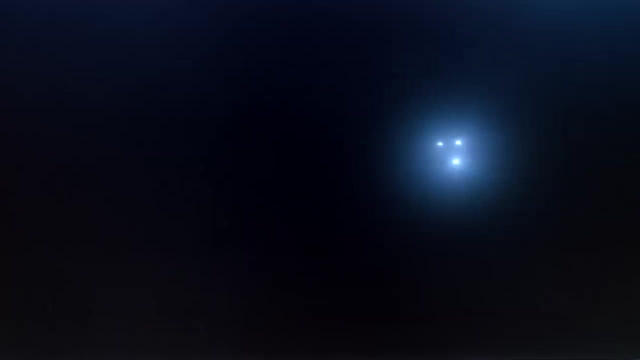 organisms with the ability to produce their own light are a few species of fungi, arthropods like fireflies, and a handful of larvae like glowworms. And while the ocean is certainly a dark place, our terrestrial world is bathed in darkness half the time too, If bioluminescence isn't in fact. 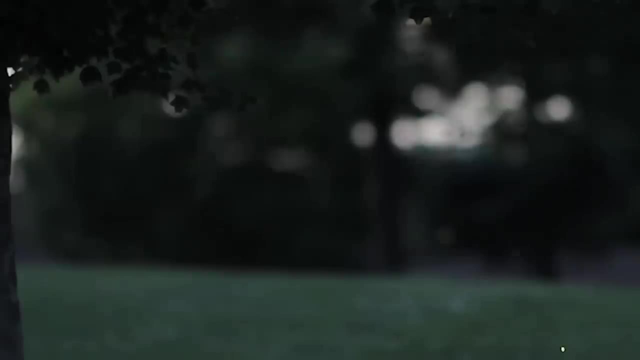 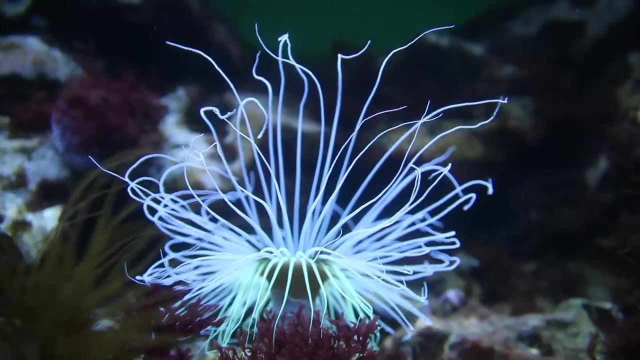 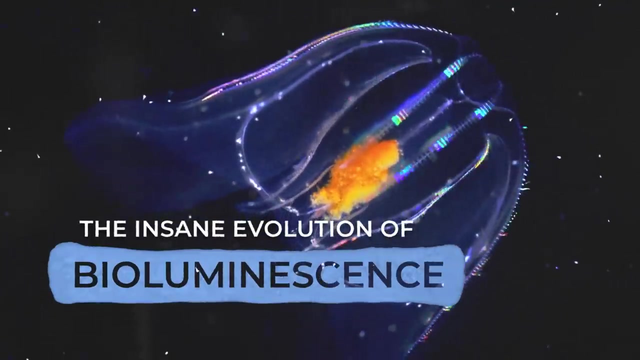 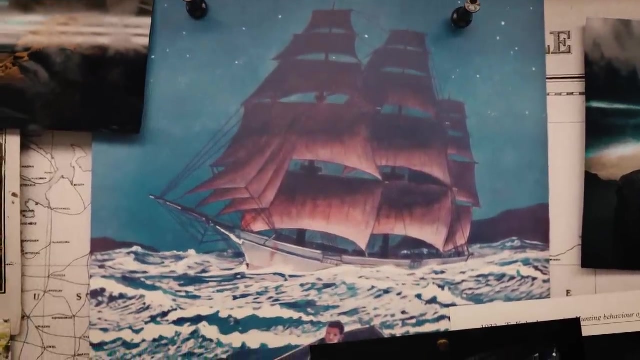 limited to the pitch black depths of the ocean? why does it seem to be constrained to barely exist on land? What is it about the world of water That makes it so much more suited to bioluminescence When 18th and 19th century travelers wrote about glowing water on the ocean? 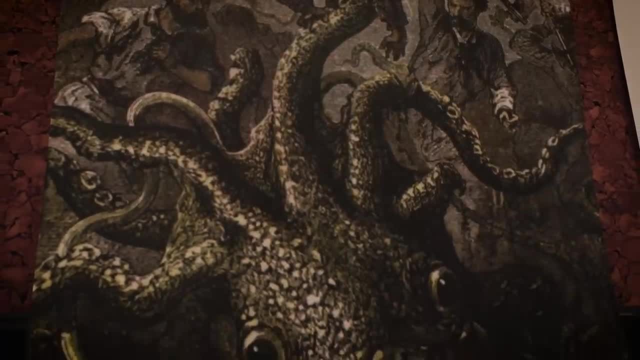 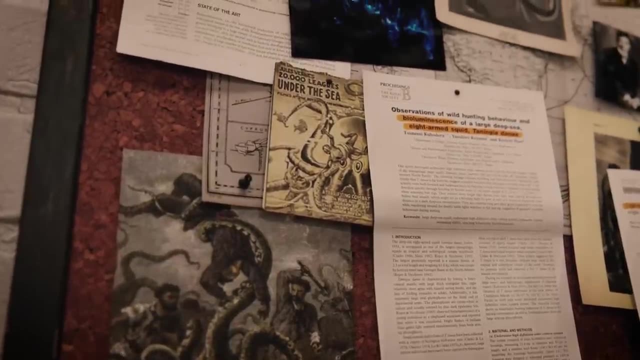 their accounts were dismissed. as fantasy, Jules Verne described a milky light coming from the ocean in his popular novel 20,000 Leagues Under the Sea. But it wasn't until the 21st century that we were able to understand that the 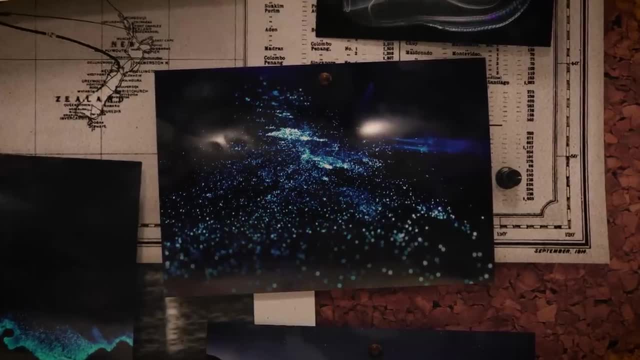 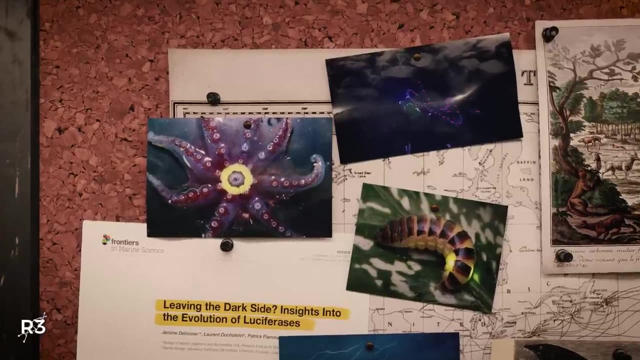 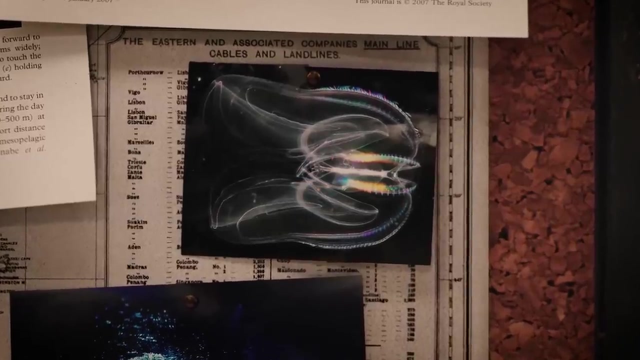 phenomenon of glowing really can illuminate huge patches of the ocean. Today, we know that bioluminescence has emerged independently more than 94 times within hundreds of species. Organisms that use bioluminescence have two options for producing their own light. They can use intrinsic bioluminescence, in which they mix chemicals. 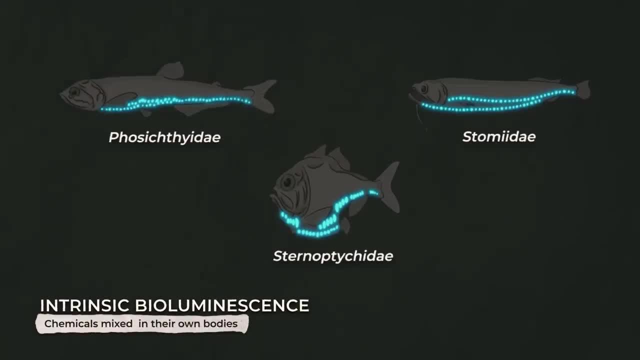 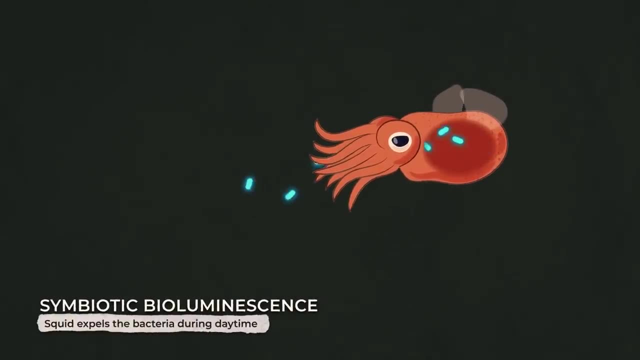 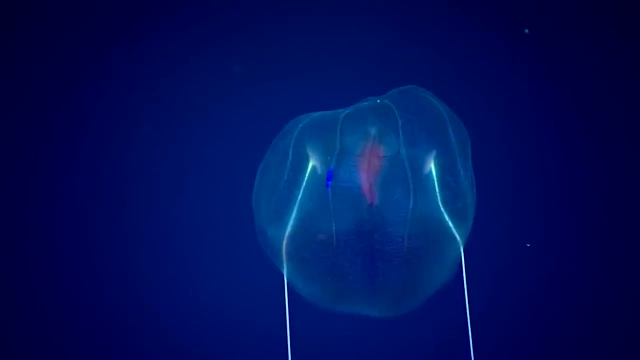 in their own bodies to produce photons of various colors and intensities, Or they can use symbiotic bioluminescence, which requires cultivating colonies of glowing bacteria in specialized organs. The chemical process involves a molecule called luciferin that generates light when mixed. 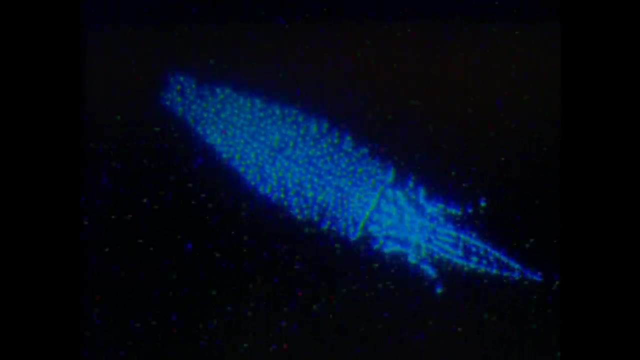 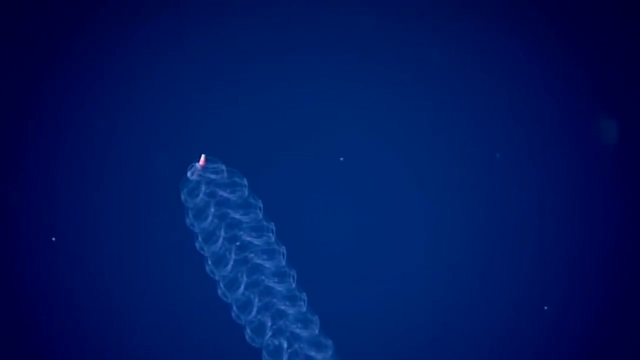 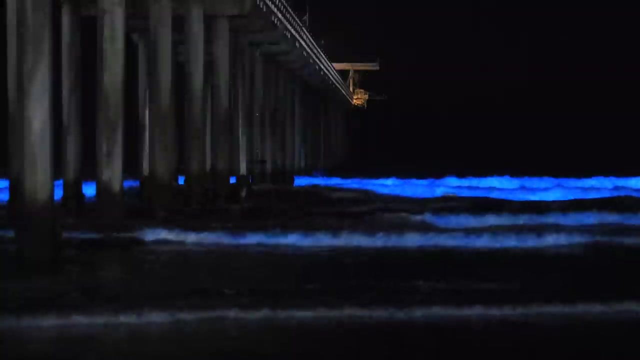 with oxygen and a luciferase enzyme. Luciferin and luciferase are generic catch-all terms. in reality, There are many different molecules that can be combined to catalyze this light-emitting reaction. This process likely originated with bacteria, and some researchers hypothesize it's. 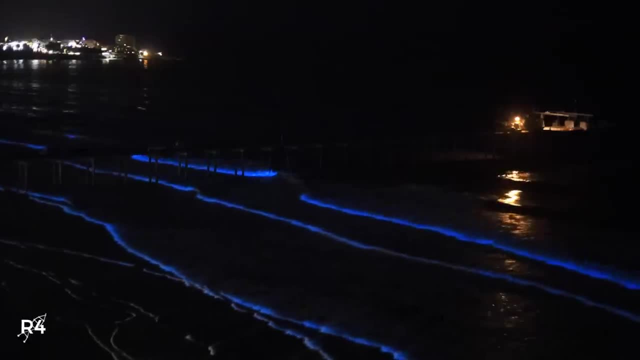 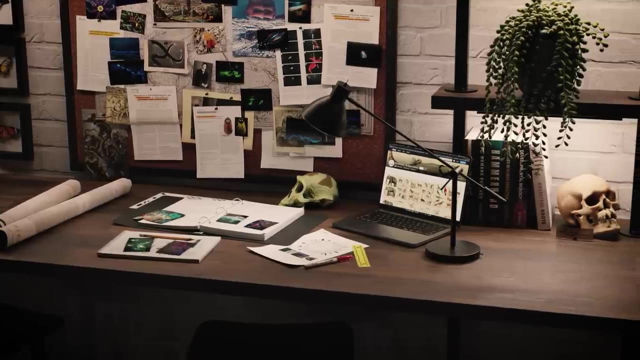 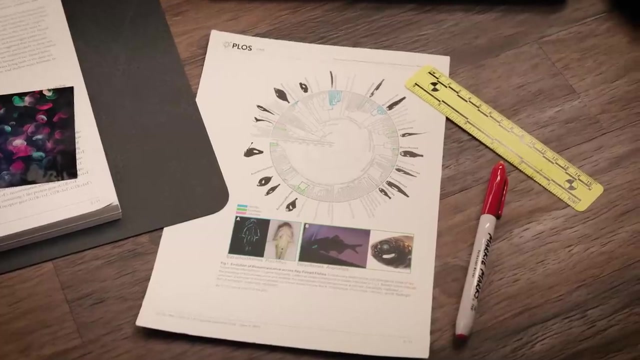 incredibly ancient. The first bioluminescence may have appeared between 2 billion and 500 million years ago. However, the two different types of bioluminescence that exist today have very different evolutionary histories. Researchers found that intrinsic bioluminescence only evolved. 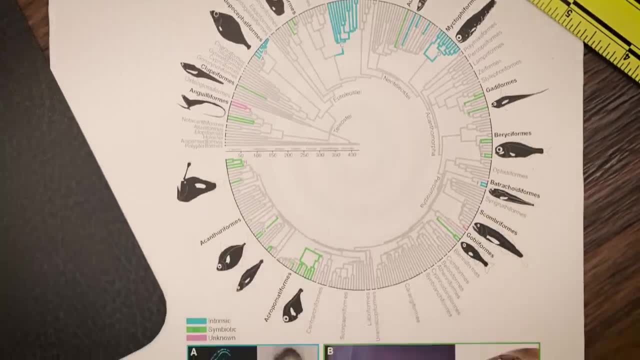 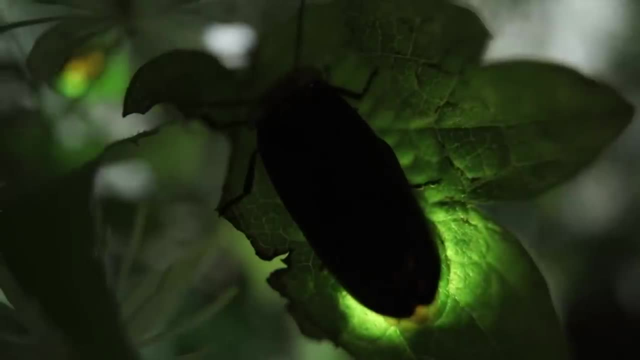 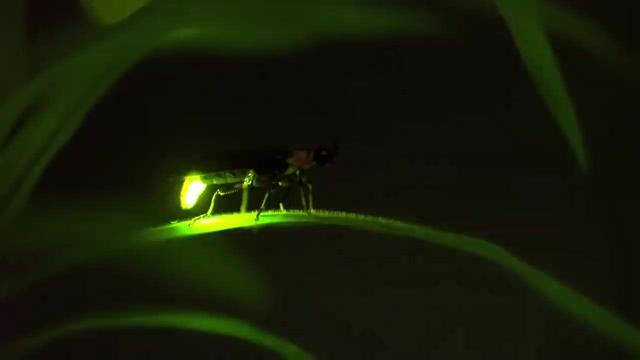 8 times in fishes, but that symbiotic bioluminescence has happened at least 17 times, always with the same family of bacteria. On land, the trait seems to have taken longer to appear. A fossilized ancestor of fireflies from 100 million years ago was discovered to have a 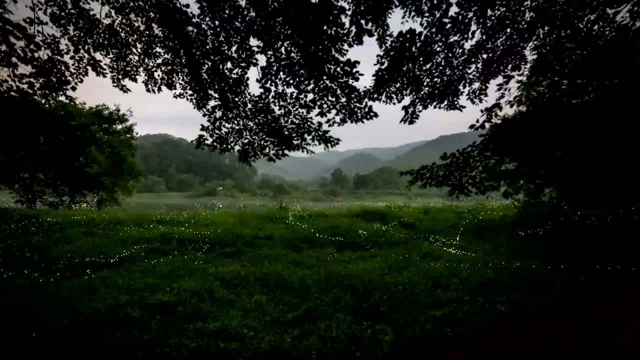 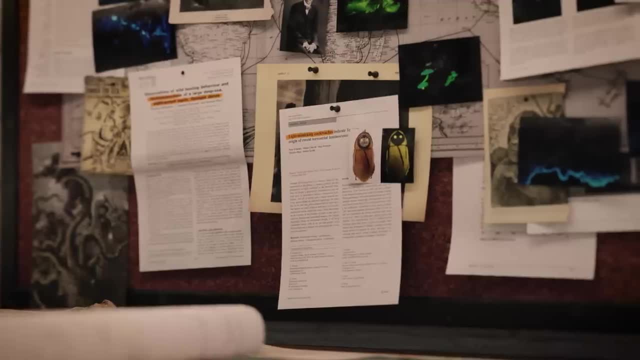 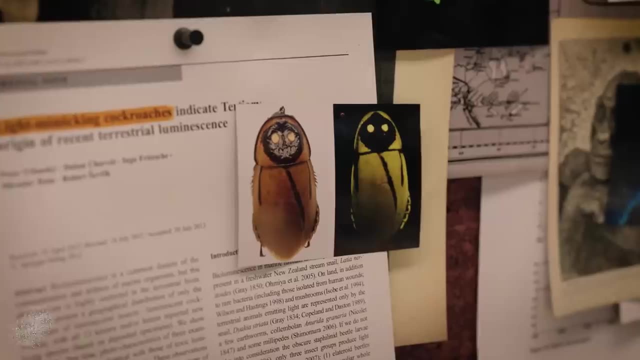 light-producing organ, suggesting that this has long been an adaptation among that group And it probably originated as a form of defense to warn off predators. Another group of researchers have suggested that other bioluminescent terrestrial insects evolved from a single ancestor that lived 65 million years ago, around the time that dinosaurs went extinct and mammals took over, But that doesn't explain fungi, since they belong to a whole other branch on the tree of life. Researchers analyzed the genome of living fungi to trace the roots of glowing mushrooms back to 160 million years ago. They theorized that 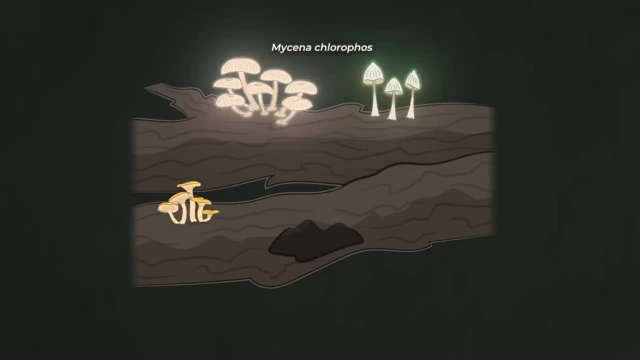 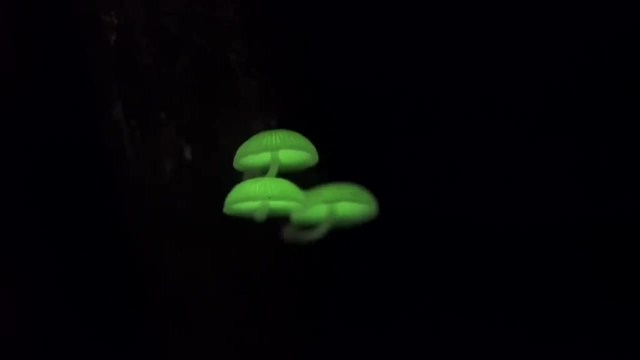 this bioluminescent ability evolved from one common ancestor that then was either lost, retained or regained across time and many different species. It's possible that the effect makes spores more attractive to insects who might spread them, But bioluminescence might. 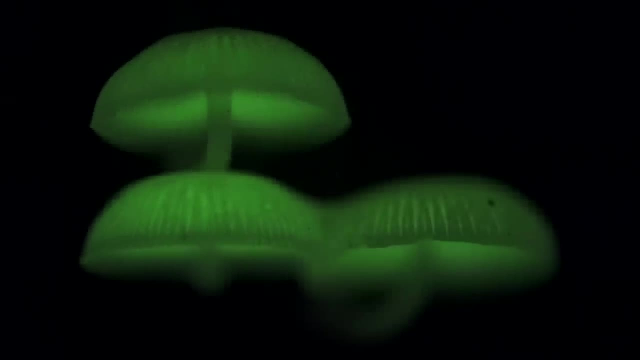 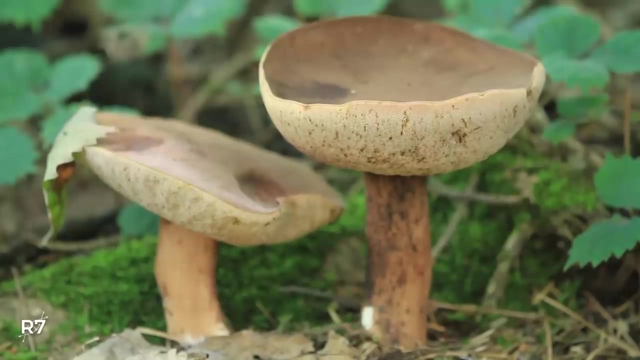 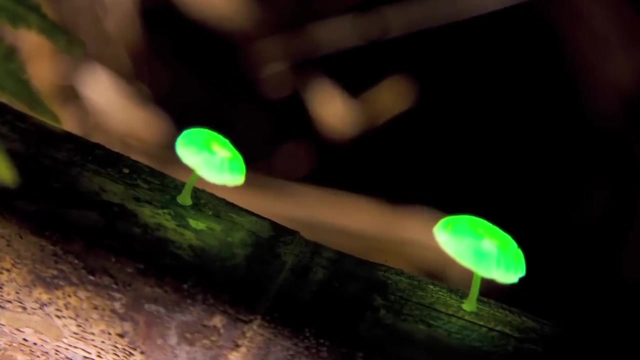 also be a byproduct of other chemical reactions, which would explain why it's disappeared multiple times through the evolutionary history of fungi. If it was serving no secondary purpose, it wouldn't need to be retained, But the fact that bioluminescence has evolved separately on land. 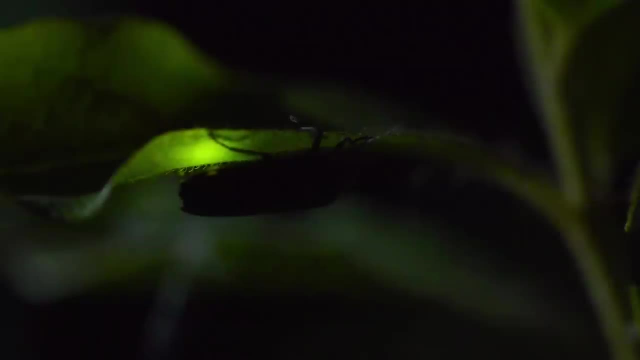 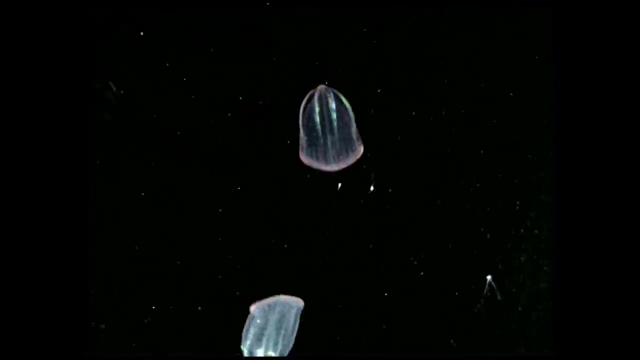 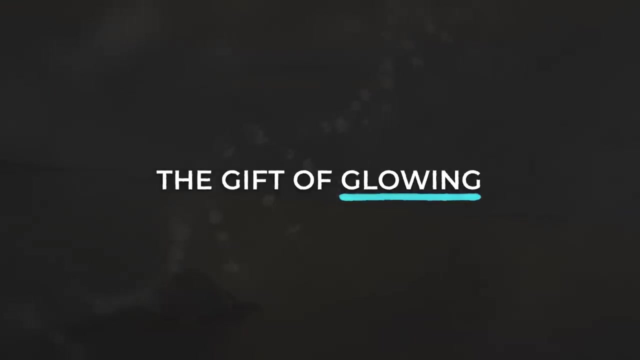 and has been retained in several species, means that it is a useful land-based adaptation. Why is it still so rare? What about the ocean? makes bioluminescence so ubiquitous? Living in the ocean is not at all like living on land. The most obvious difference between 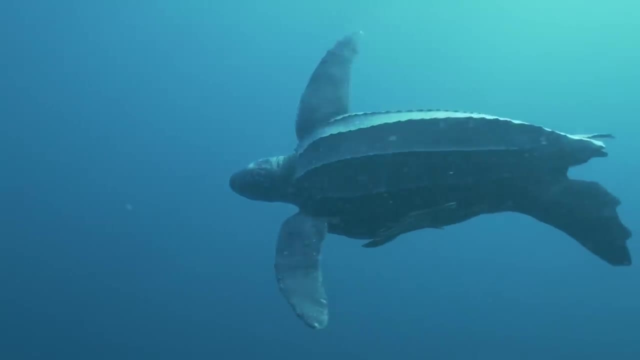 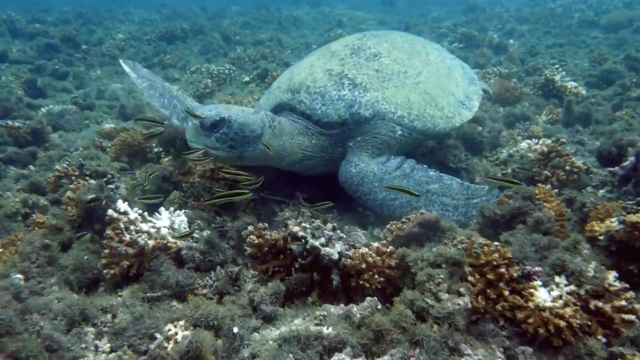 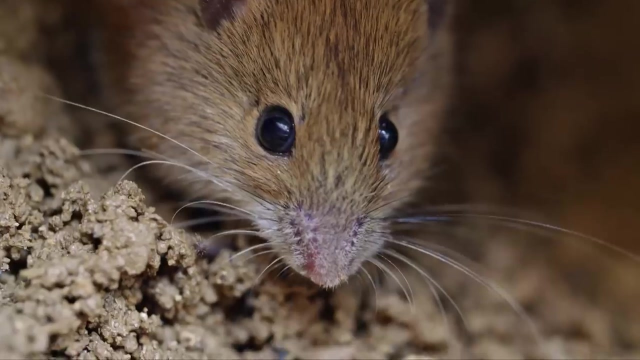 marine and terrestrial environments is the medium: water versus air. Both present vastly different challenges and opportunities to lifeforms who live in them. But a less obvious difference is the fact that in most of the ocean there's nowhere to hide Rodents and other small 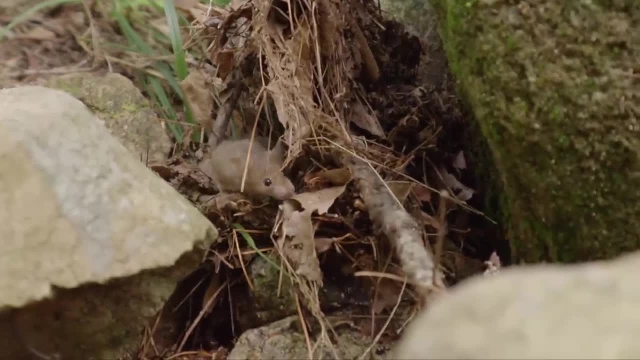 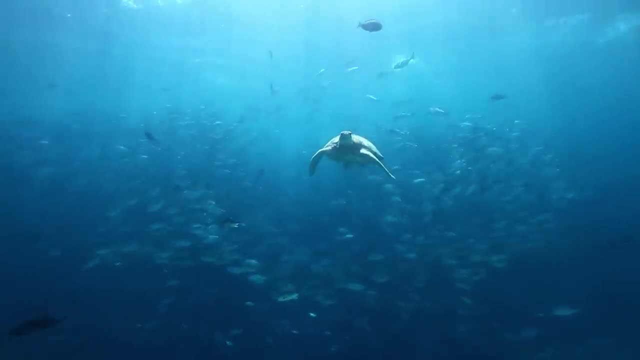 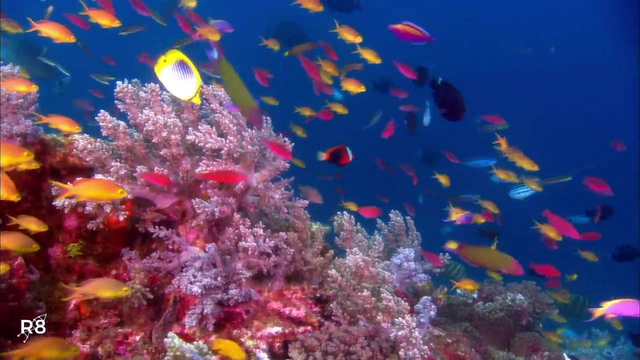 animals on land have trees, shrubs, rocks and burrows that help them stay safe from predators. Meanwhile, for most aquatic life, there's nothing in the environment to keep them safe. Reef systems are the exception rather than the rule. They only occur in about 1% of the ocean. 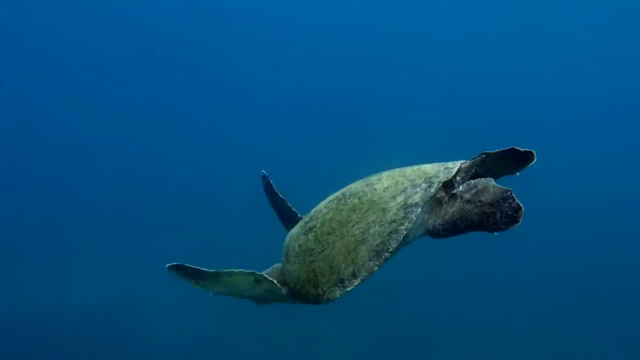 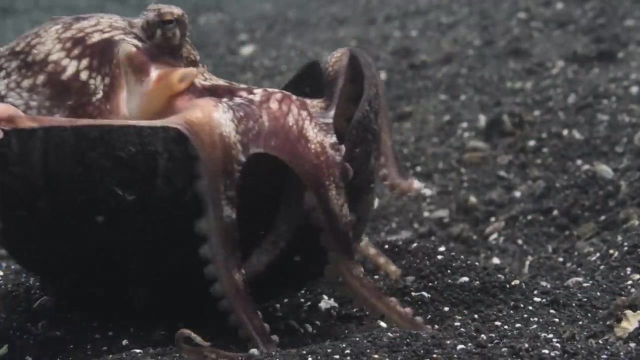 and only some species live on the ocean's floor. Nearly everywhere else in the ocean is an open expanse. That means many species have had to find other ways of keeping themselves safe from predators and, as unexpected as it might be, light is one of the best methods. 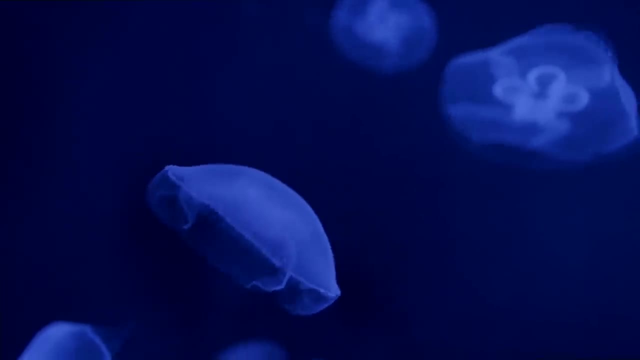 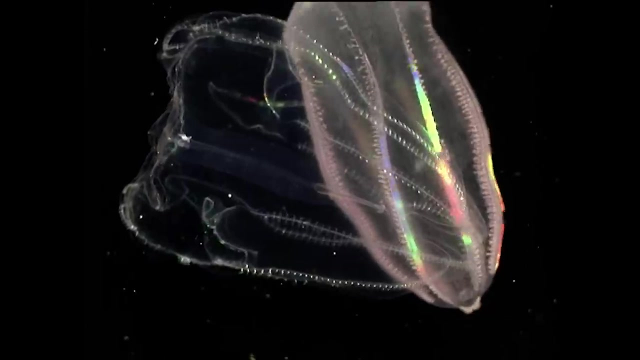 Jellyfish and siphonophores are some of the best examples of creatures that use light to evade capture. Nearly all of them have some form of bioluminescence Comb. jellies flash brightly to startle predators, while siphonophores can produce a constellation of small lights. 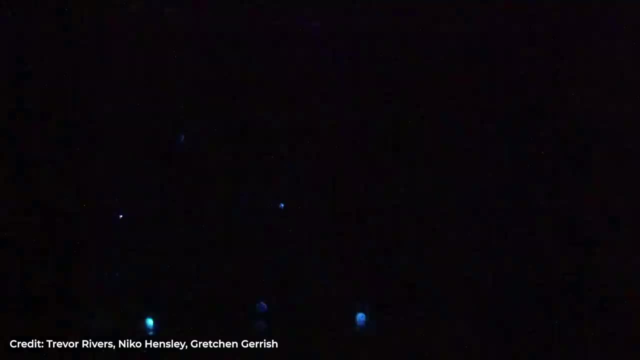 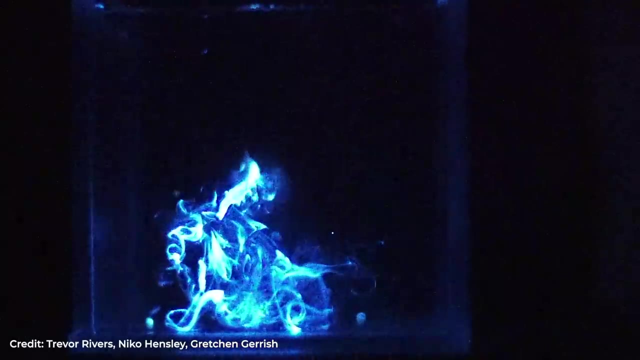 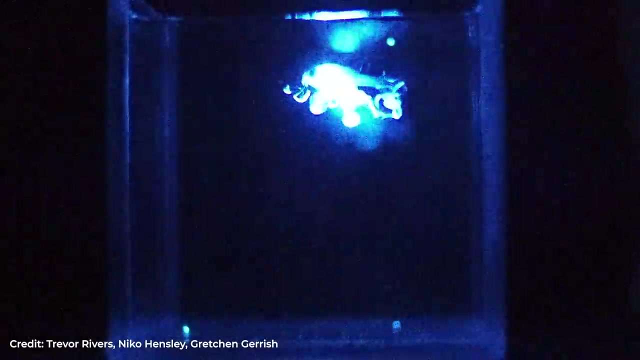 Mimicking plankton. to confuse predators, Some jellies even release a glowing slime that sticks to their predator, a strategy also employed by tiny crustaceans called ostracods or sea fireflies. When fish try to swallow them, they release one of the brightest lights in the ocean. 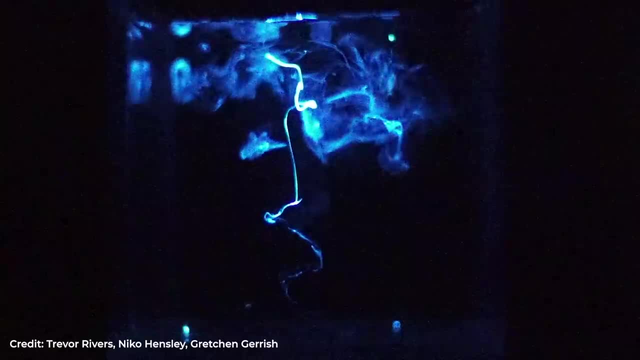 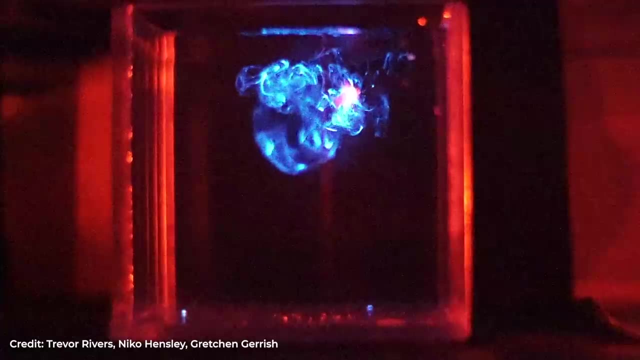 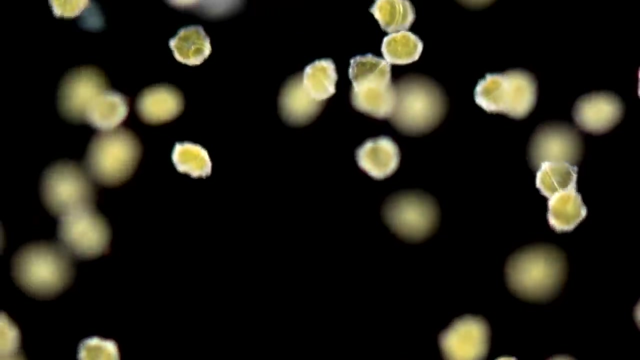 momentarily blinding the fish and smearing it with light By illuminating themselves or their predator. these organisms might also be calling over and even larger predator- The ones who might eat the smaller organisms- would be predator. Consider dinoflagellates, those single-celled plankton that can produce. 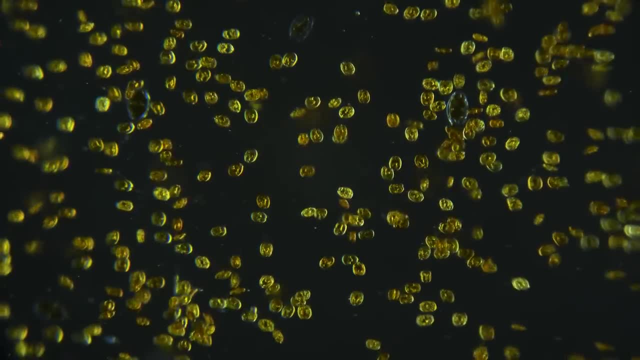 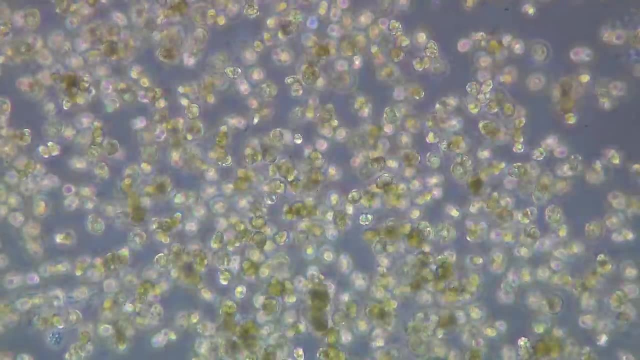 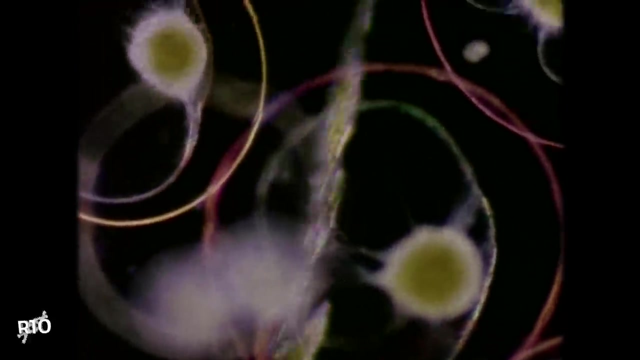 such wonderfully glowing waves. There are many species of dinoflagellates, and those that are capable of bioluminescence are less likely to be eaten. This could be because their bright flashes act like a burglar alarm, essentially announcing to the nearby ocean dwellers: hey, this crystal. 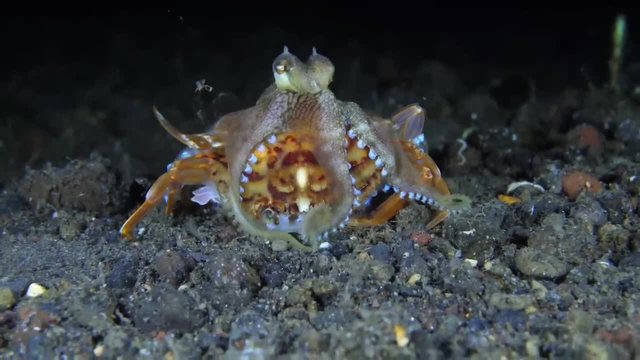 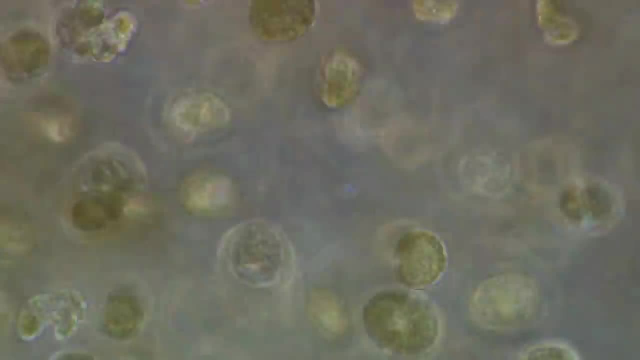 station is trying to eat me. You wanna come eat him? The last way swimmers use light as a source of defense sounds the most counterintuitive: light as camouflage. The deeper you go in the ocean, the less light filters down through all. 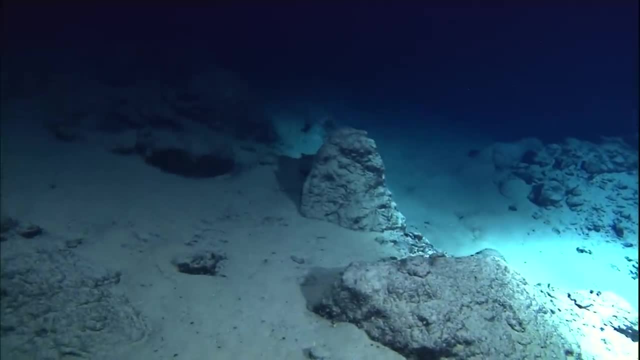 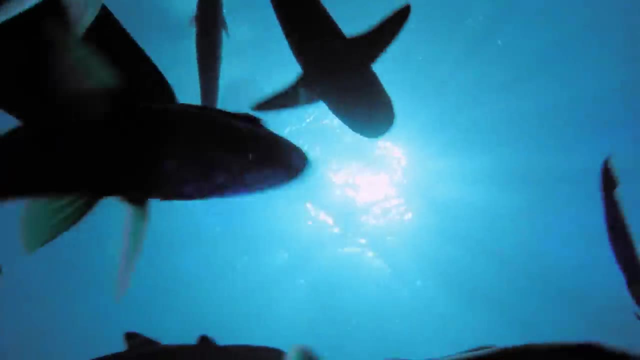 that water, Between 200 meters and a thousand meters, lies the mesopelagic, also known as the twilight zone, Because a certain amount of light does come from above. a fish swimming above a predator would have its dark silhouette out of the water and the fish would not be able to see it. Mimicking plankton to confuse predators. Some jellies even release a glowing slime that sticks to their predator, a strategy also employed by tiny crustaceans called ostracods or sea fireflies. Mimicking plankton to confuse predators. These organisms might also be calling over and over again. 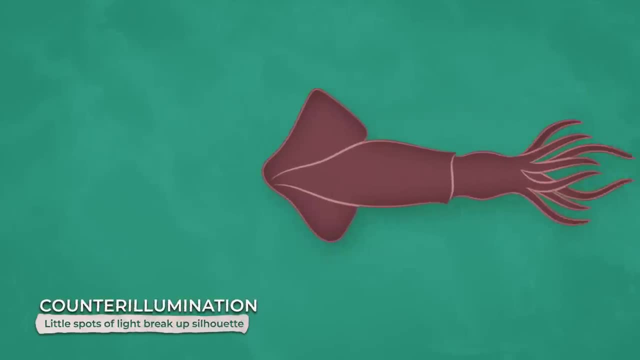 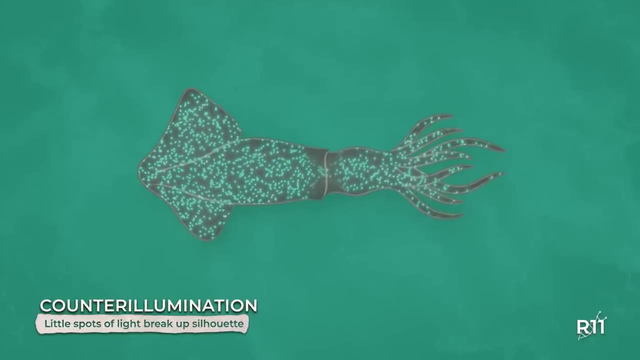 outlining against the light. To keep this from happening, they use counter-illumination. Little spots of light on their underside break up their silhouette, confusing potential predators. It's such a well-honed trick that creatures like the Hawaiian bobtail squid can change the 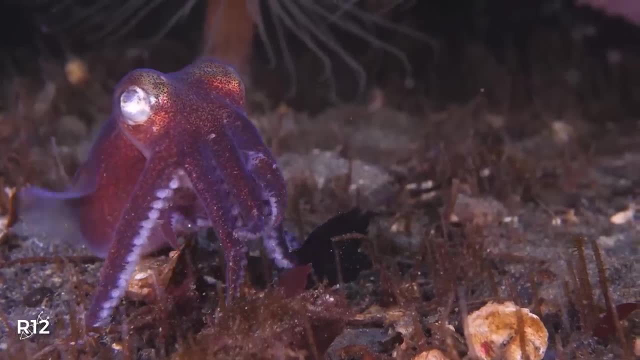 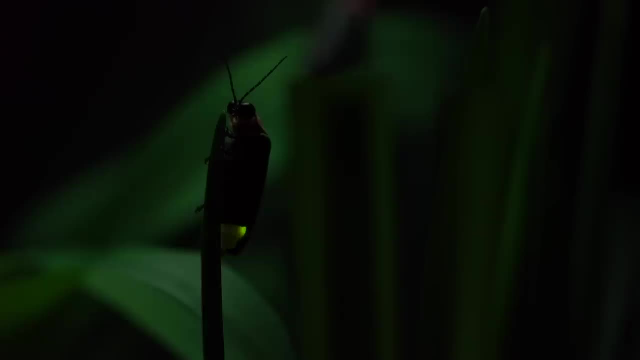 amount of light it emits, depending on the time of day, like its own glowing circadian rhythm. The story on land is a little more complicated, since lighting up in the darkness is more likely to draw attention to you than it is to the other side of the ocean You might want to. 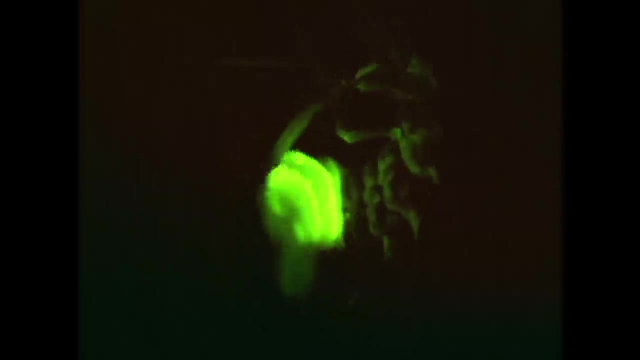 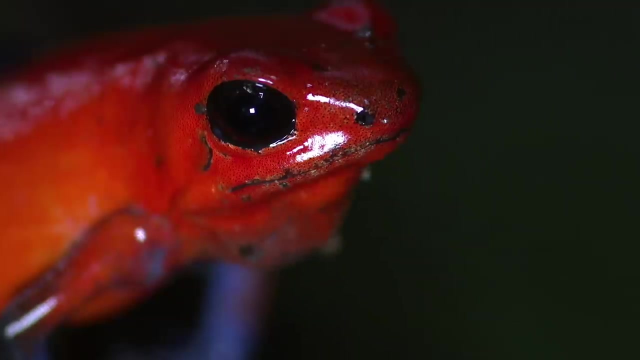 make sure that the light is as bright as possible so that you can see it better. But this glow can still be a defensive strategy for some organisms by advertising that they are poisonous. It's like a nighttime version of the poison dart frog's vibrant skin color. 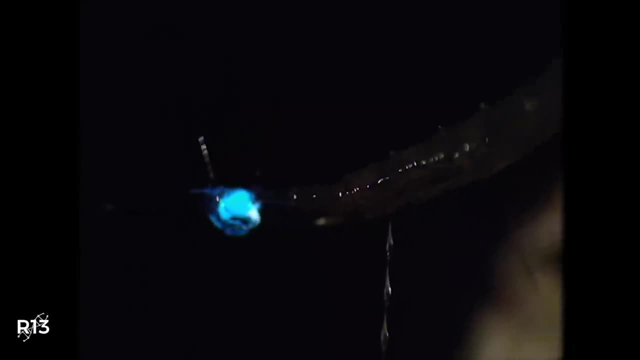 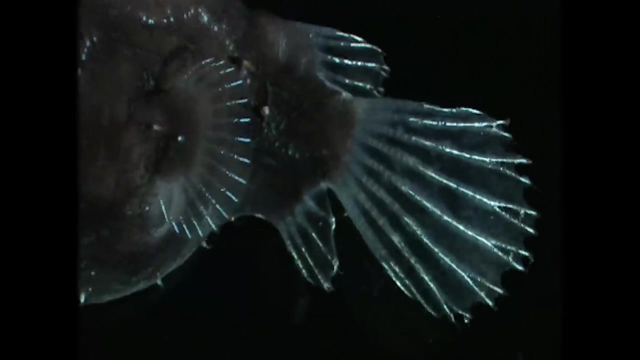 This strategy is used by some worms as well as millipedes, But of course it's not only prey who are using light to keep themselves alive. Predators have many of their own tricks to lure in their meals. Members of the anglerfish family. 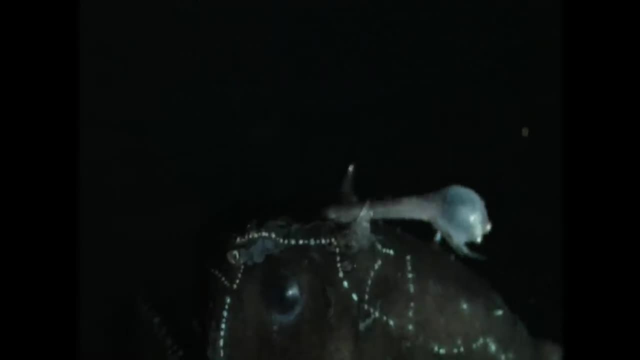 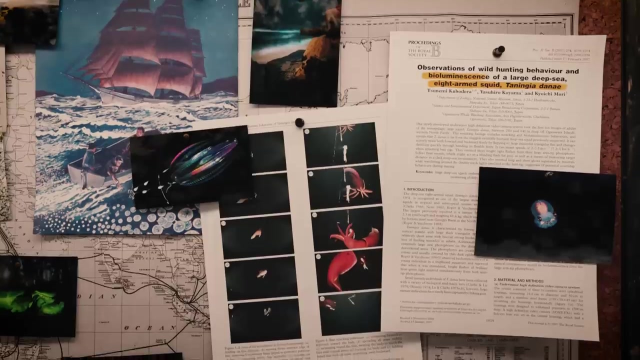 might be the best-known deep-sea dwellers to entrance their prey with glowing lures, But the strategy also seems to be used by giant squid, who have been observed flashing bright lights while hunting, either as a way of stunning their prey or getting them to come closer. 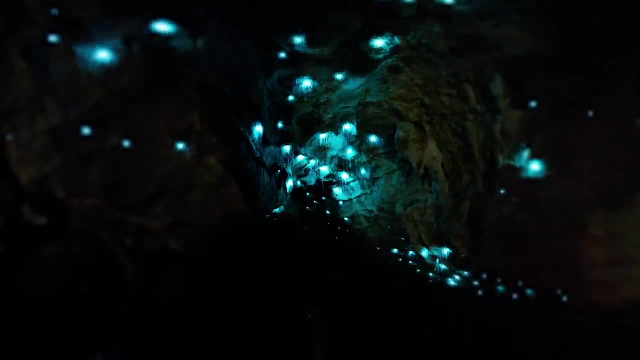 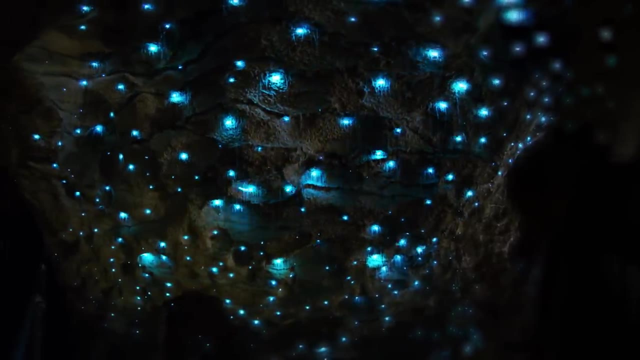 And this hunting technique is something shared among many of the bioluminescent insects that glow on land. Consider the glowworms that have enchanted people for centuries in Australia and New Zealand. These cave-in-the-dark bioluminescent insects are the only ones who have been able to. 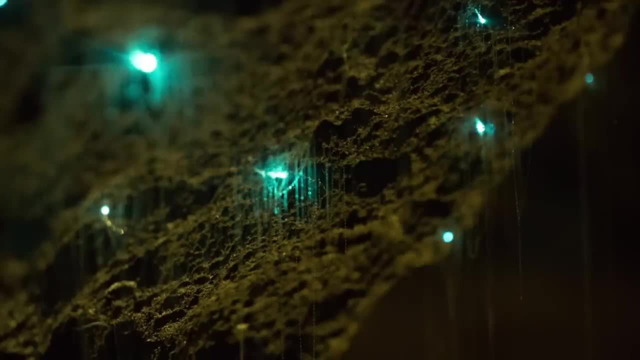 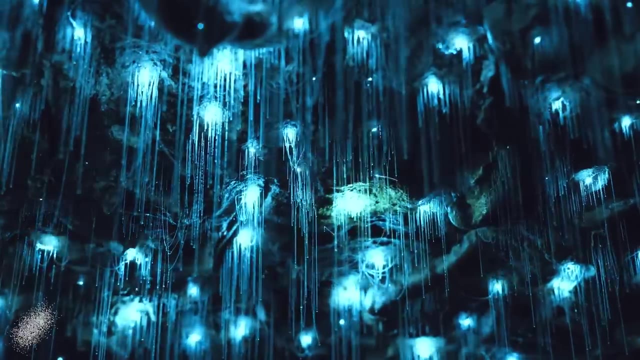 get close to their prey. They are also known as the giant squid, which is one of the most popular species in the world. These cave-dwellers fill the ceilings of their abodes with starry blue constellations, But that light is actually a creepy hunting strategy. The worms spin. 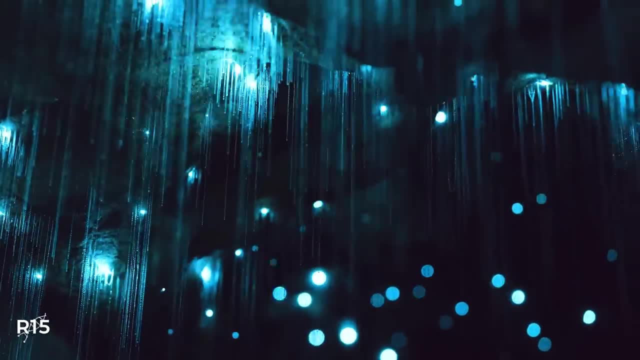 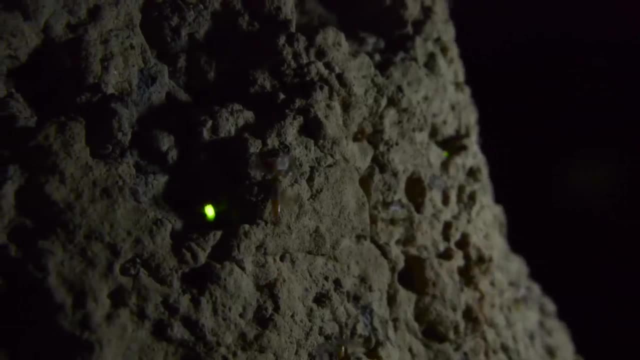 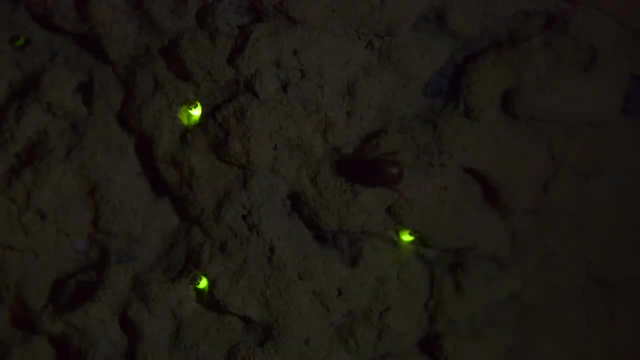 dripping nets of glowing spit into which other insects fly. The larvae of click beetles operate very similarly, hiding in holes and emitting a soft yellow-green glow. Whenever insects approach to investigate, the beetles' pincers snap shut around its meal, Just like in the sea organisms. 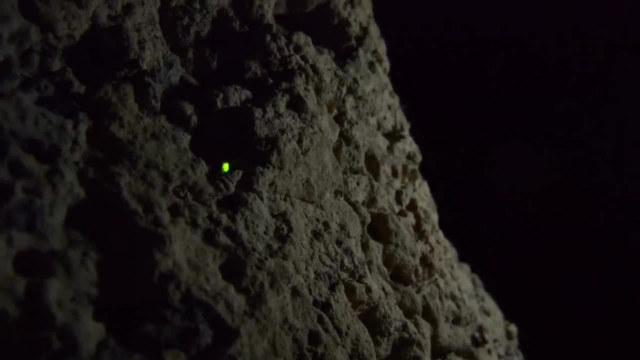 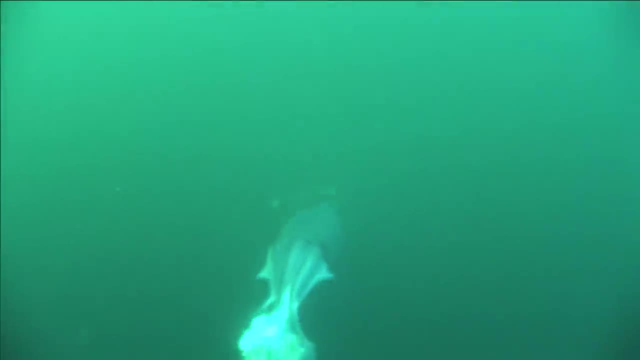 on land have been able to turn bioluminescence to their advantage when it comes to hunting, But perhaps the most mysterious use of bioluminescence is light for mating and communication. Scientists recently discovered that the Humboldt squid a voracious hunter. 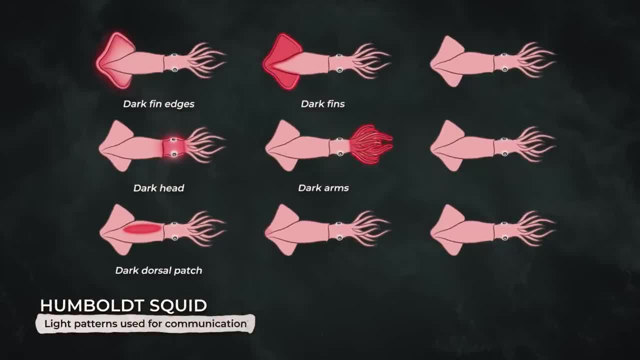 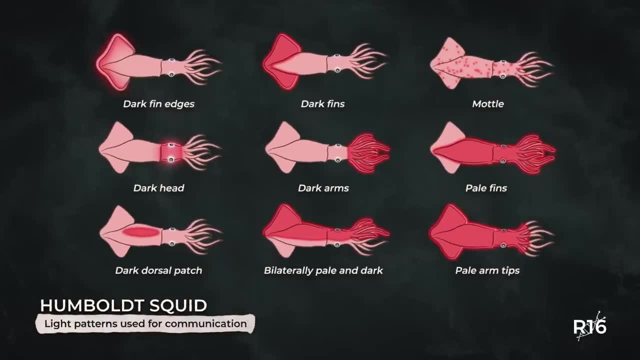 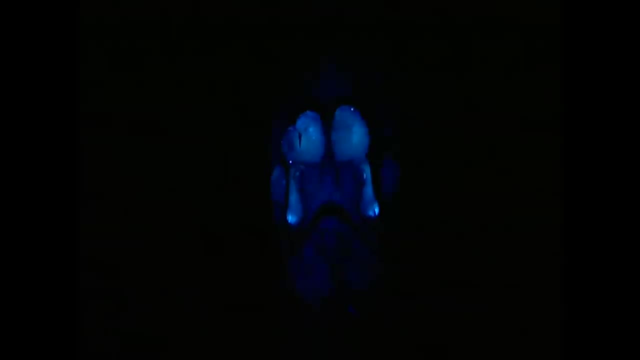 uses a number of different light patterns depending on the context it's in. These changes might reflect messages that they're communicating to other squid, whether it's dominance displays or claiming certain prey. And then there's also the case of lanternfishes, which include more than 250 species swimming. 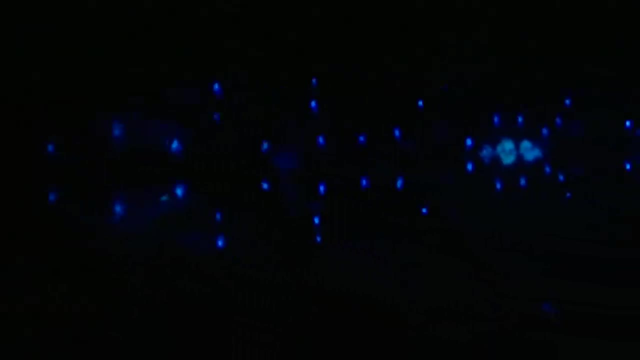 around the Mesopelagic. In addition to having lights on their stomachs for camouflage purposes, they also have glowing spots on the sides of their heads. Researchers have hypothesized that different species have subtly different glowing signals they use to find mates. If it's a strategy that sounds familiar, it might be because so many of us have watched. 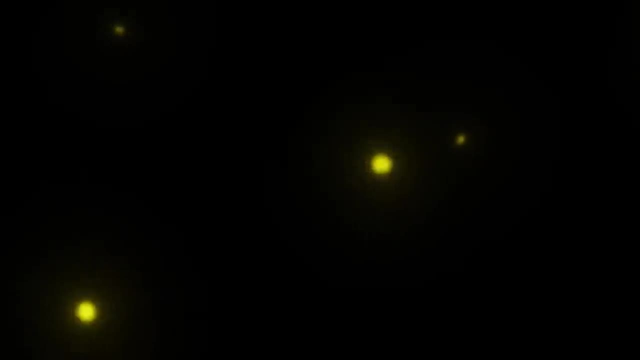 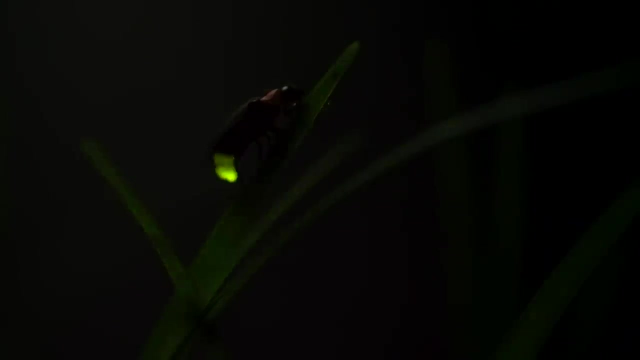 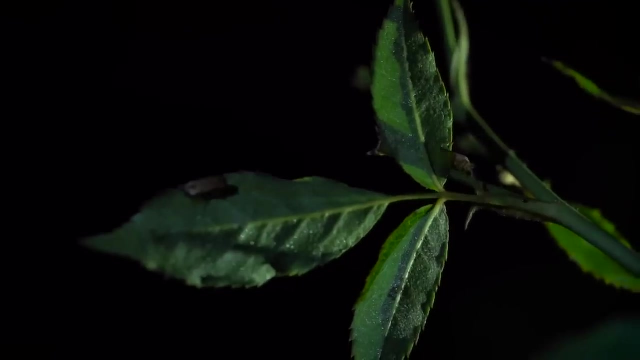 lightning bugs dance through the darkness on summer nights nights. These flying beetles also use bioluminescence for mating purposes, with different species flashing at different intervals to attract mates. But still, light-up displays like firefly dances are the exception, not the rule for life on land. 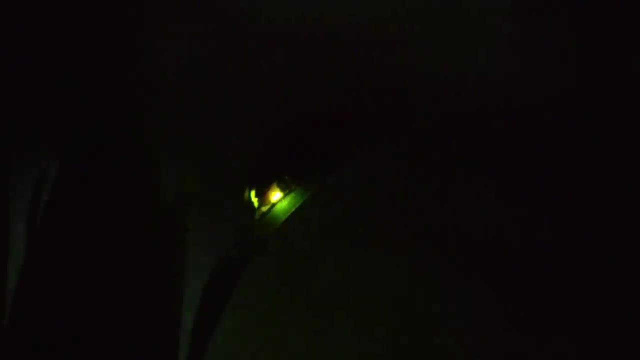 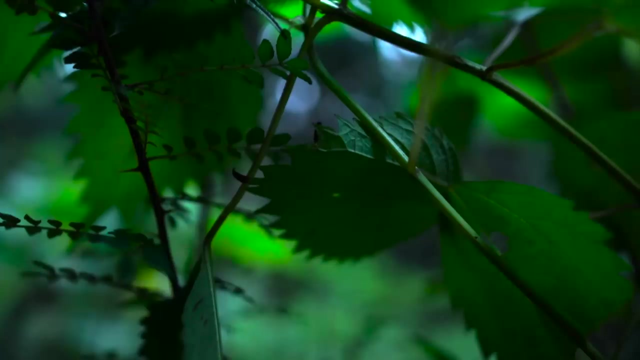 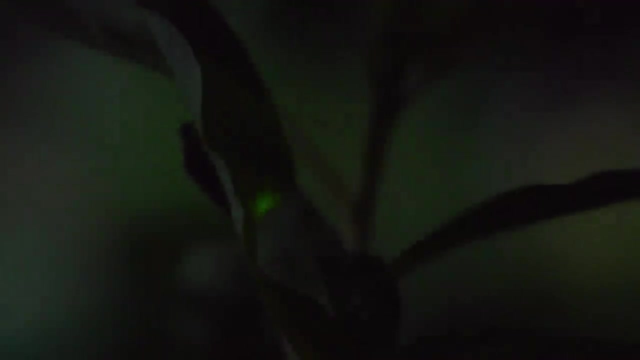 Despite its clear utility for some creatures, researchers think that it might be harder for terrestrial life to develop bioluminescence because the chemicals involved can be quite toxic and might be harder to cleanse away when the creatures aren't always swimming through water. But this toxicity is unlikely to be the full story as to why bioluminescence. 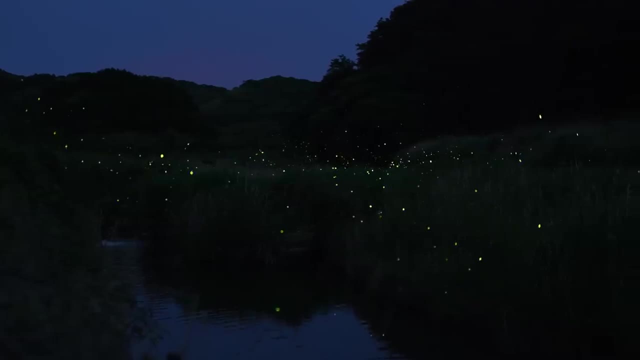 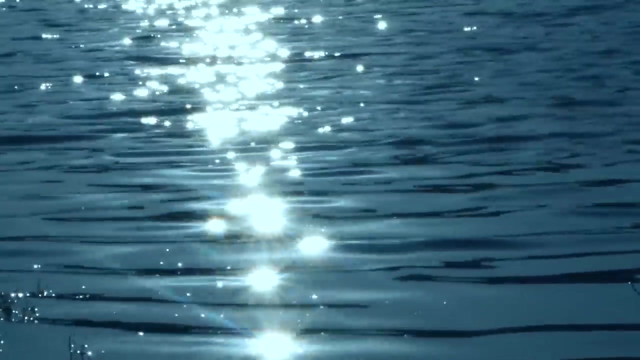 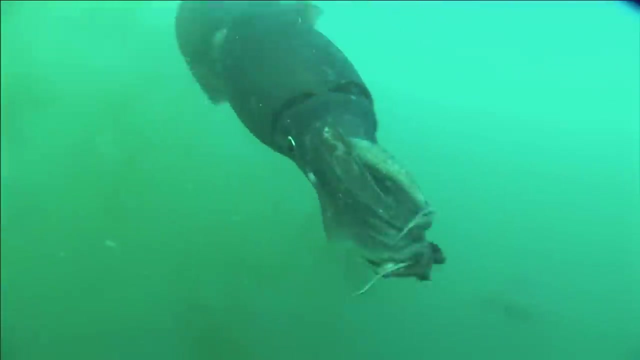 isn't more common on land, since bioluminescence is also basically non-existent in fresh water, where toxicity could be removed, as well as in the ocean? The answer perhaps has to do with something simpler: time Life hasn't existed on land and in fresh water as long. 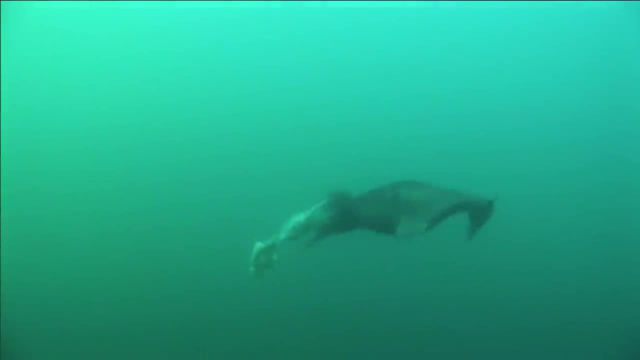 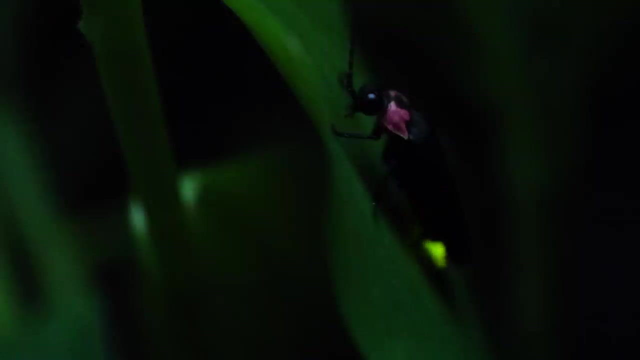 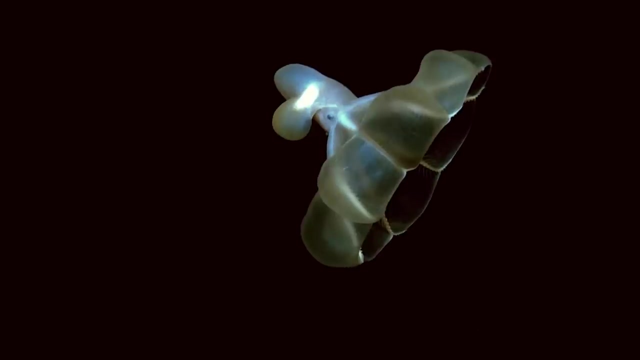 as it has been, And evolution is a slow process. Perhaps it's not that land-based organisms don't have bioluminescence, it's that they don't have bioluminescence yet. It's clear that we have a lot of work yet to do to understand the past and future of 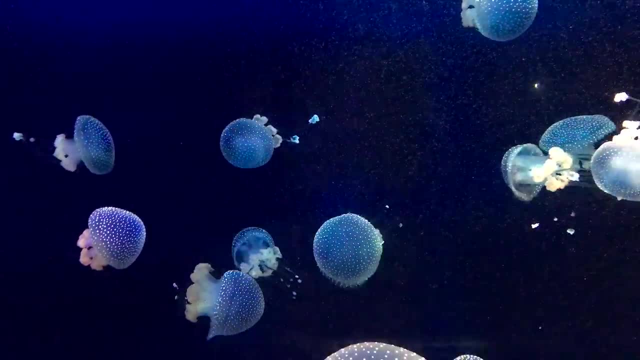 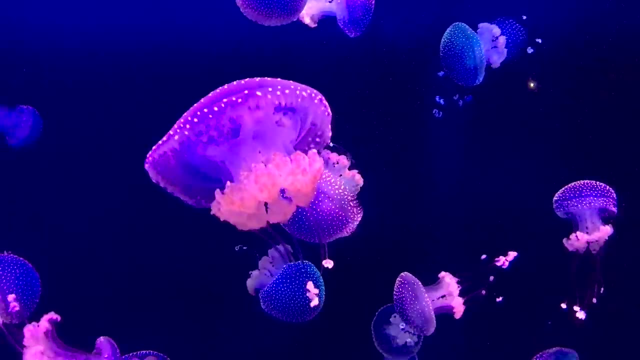 bioluminescence, But if we ever make it far enough into the universe to discover life on other planets, scientists say we should be on the lookout for bioluminescence, Because where there's water and air there's a pretty good chance we'll find lots of glowing.